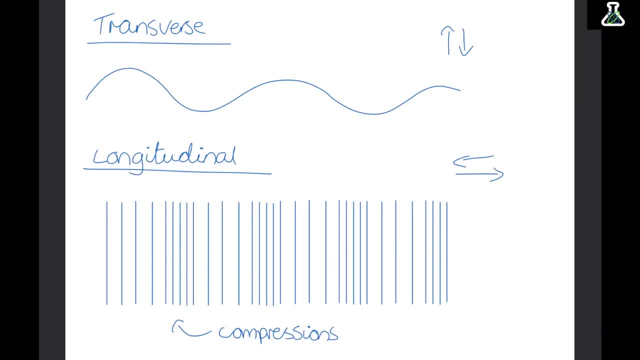 compressions, which is when the vibrations are close together, andningar and error-fractions, which is when the vibrations are far apart. Now, a wavelength is still measured from one compression to another compression. Now, some examples of transverse waves are light waves, water waves at the beach and all waves on the electromagnetic spectrum. 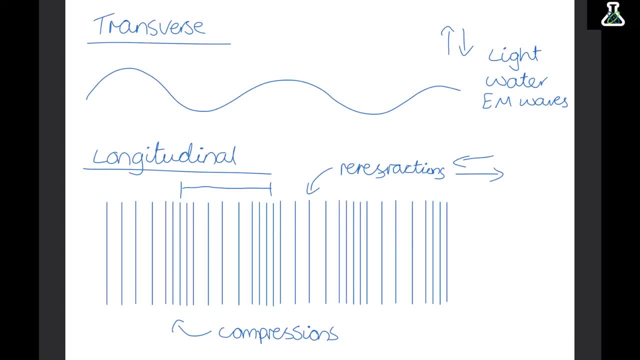 And we'll look at those waves later. Now some examples of longitudinal waves are sound waves and pea waves, waves which are a type of seismic waves that are to do with earthquakes. Now, a sound wave with a high pitch just has very short wavelengths, so the compressions 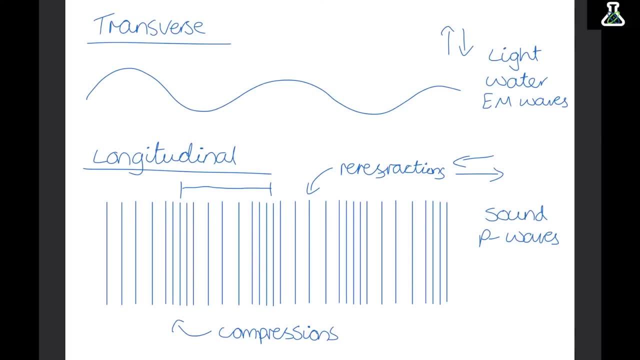 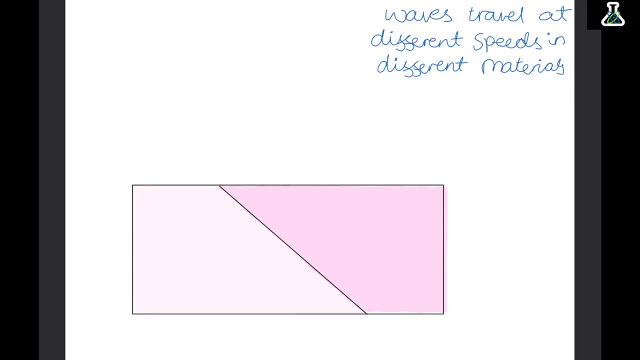 are really close together and sound with a low pitch has really long wavelengths. Now, waves travel at different speeds in different materials, and when the material or wave is travelling in changes. three things can happen. A wave can be transmitted, which is when it passes through the material absorbed, which 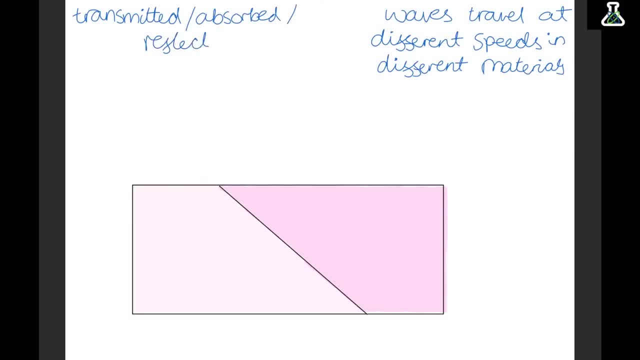 is when the object just simply absorbs the wave, or reflected, which is when the wave bounces back off the material. Now we're going to look at a type of transmission, and this is refraction. So let's say that in this diagram the light pink side is air and the dark pink side is 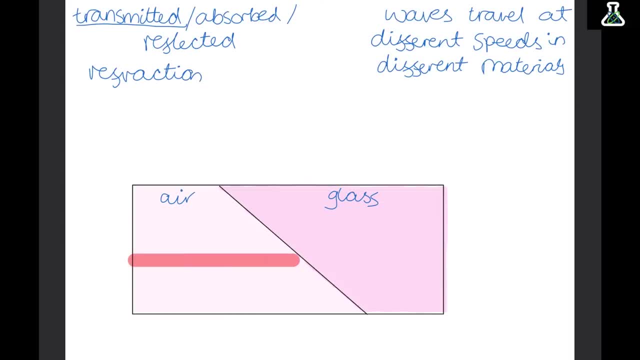 glass. Now imagine a light wave travelling towards the glass at an angle. Now this side of the light wave hits the glass first, so this is going to slow down and change speed first. Now this side is still travelling at a normal speed, so this is going to change speed last. 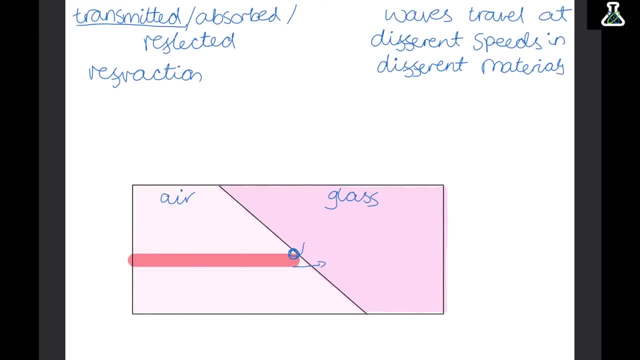 Now, as this changes first, Then this is still going and this pulls the wave around in this direction and starts travelling at an angle through the glass. Now, this change of direction is called refraction. Now, when this happens, the frequency of the wave doesn't change. 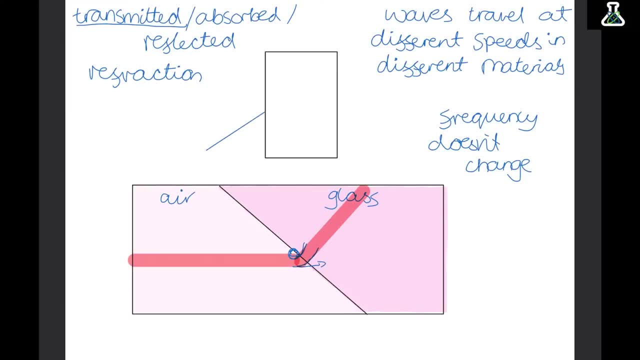 Now we can draw diagrams to show refraction happening, So we can draw the wave coming in to the new material and then the change of direction. There are two angles that we can measure from this. we can measure the angle of incidence and the angle of refraction. 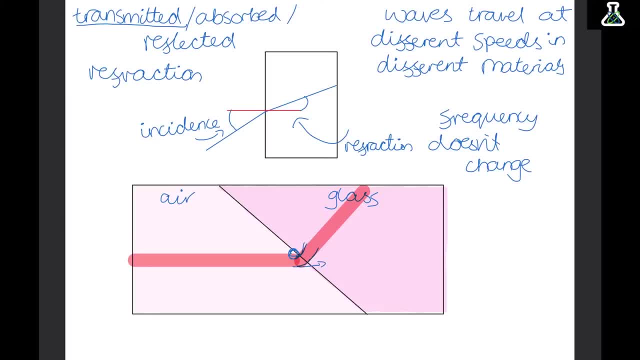 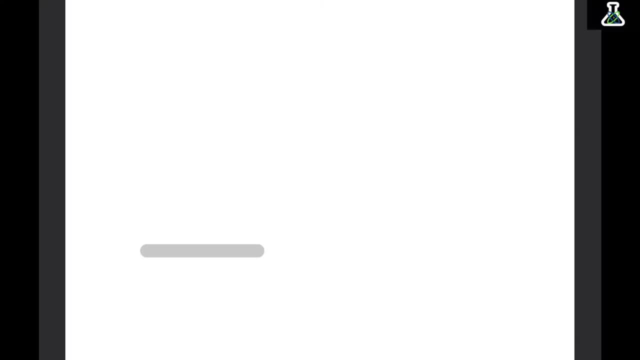 So the angle of incidence is just the angle that the wave enters the new material, and the angle of refraction is how much the wave has changed direction. Ok, so we also said that when waves hit a boundary they can be reflected. So as a wave comes in to a new material- so say this new material is glass- they can bounce. 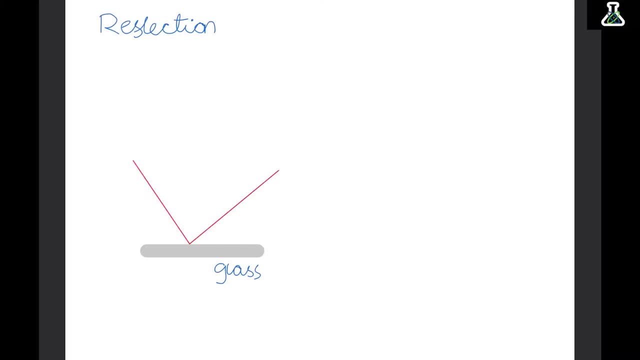 straight back off, and this is called reflection. When you look in a mirror, the light waves are coming from the light source hitting you, hitting the mirror and then bouncing back off into your eye so you can see yourself. Now the angle of incidence and the angle of reflection are always equal. 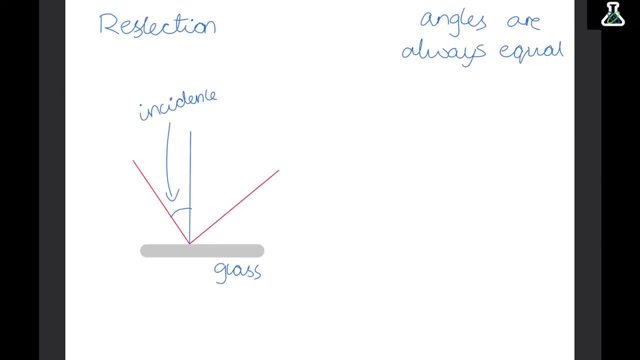 So here is the angle of incidence. Again, this is just the angle that the wave came in to the new material. Now here is the angle of reflection and this is the angle that it bounces back off of the material. at Now, these angles will always be equal. 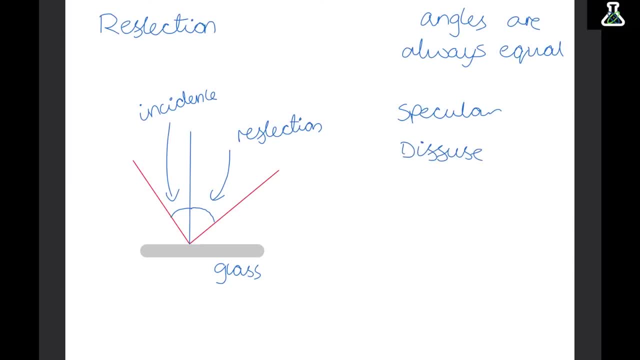 Now, reflection can be specular or diffused. Ok, Now this is an example of specular reflection, So the surface is completely flat, so all of the light waves can bounce off uniformly. But diffused reflection is when the surface is uneven or rough, So as each light wave comes in they all hit different points, so they are all reflected. 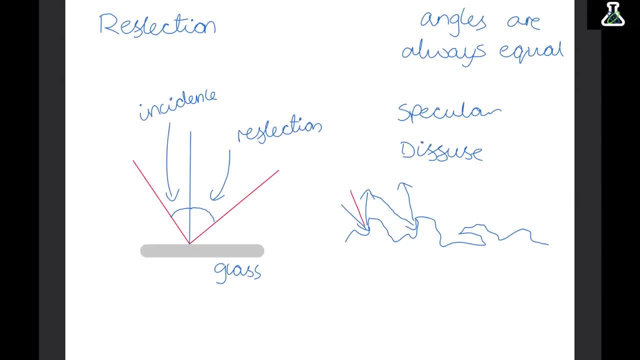 at different angles. Although the angle of incidence and reflection will always be the same For every light wave, they are going in different directions because they have all hit different points. Now, it's not just light waves that can be reflected. All types of waves can. 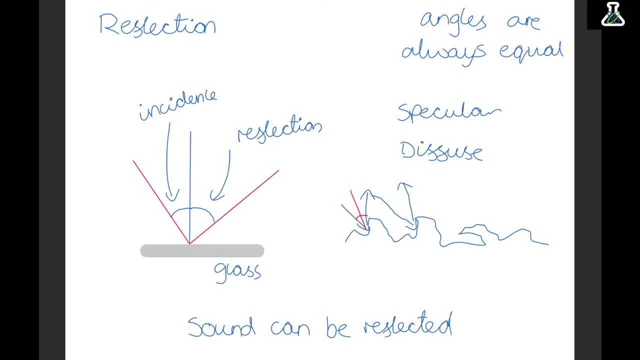 And a useful one is sound waves. So if we use really really high pitched sounds, we can fire them at things and they will be reflected straight back. and this is ultrasound And this is useful for loads of different things. We can use it to create pictures of babies in the womb. 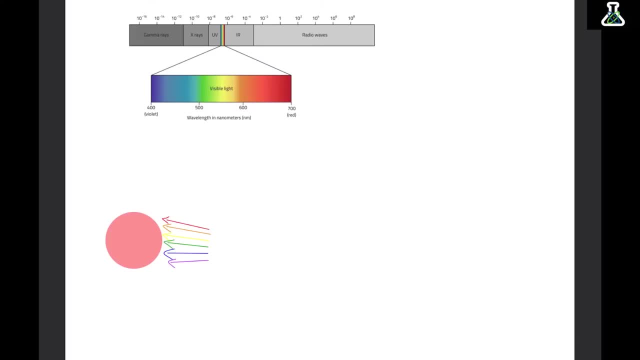 Ok, So now we are going to look at the electromagnetic field. Ok, So this is the electromagnetic spectrum. Now, this is the electromagnetic spectrum. It's a range of all transverse waves depending on their frequency. Now, this also shows visible light. 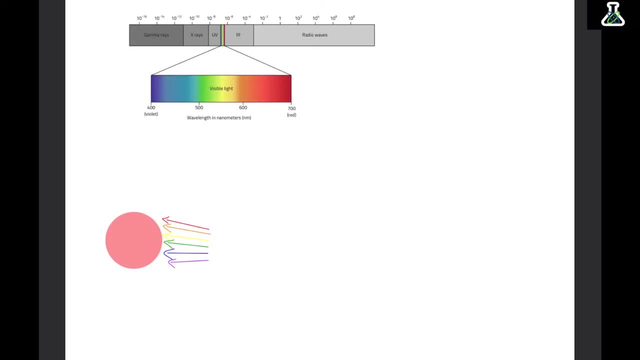 And this makes up a small part of the electromagnetic spectrum and it's the only part that human senses can detect. So red light has a really low frequency. Blue light has a really high frequency. Now, it's also really important that you know that all of the colours on the spectrum of light